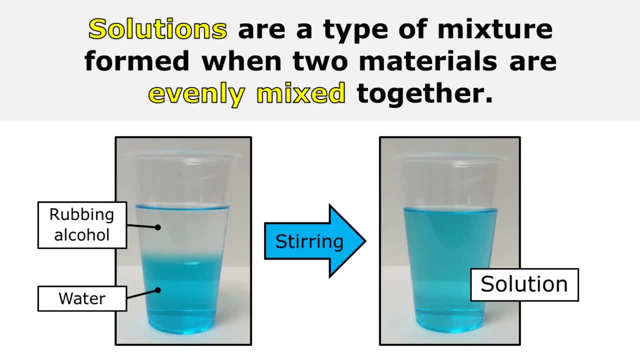 substances that have been mixed together. Solutions are a type of mixture formed when two materials are evenly mixed together. So on the left you can see that I've got some water and some rubbing alcohol in the same cup. Now rubbing alcohol and water are both clear liquids, so I put some blue dye in the 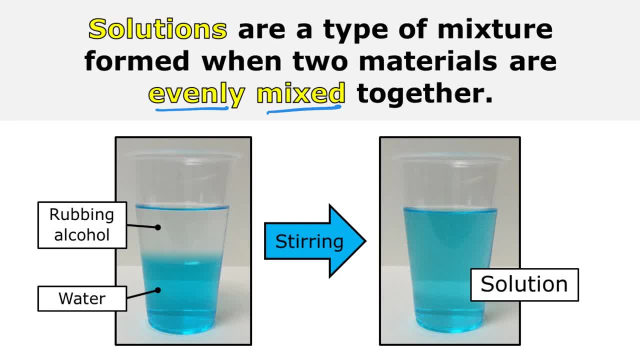 water so that you could tell them apart. But you can see that they're not evenly mixed yet. But once I stir these two liquids together, I create a solution. The rubbing alcohol and the water have been evenly mixed together, and so that is what makes a solution. Liquid solutions are often 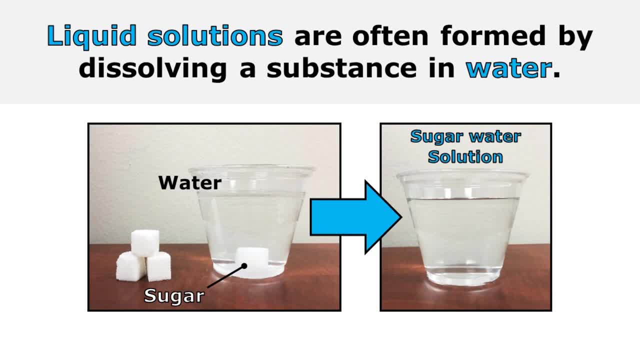 formed by dissolving a substance in water. So you can see here that I've got sugar cubes and water and there's already a cube of sugar at the bottom of that cup of water. After a while that sugar completely dissolves and becomes evenly mixed with the water and that creates a 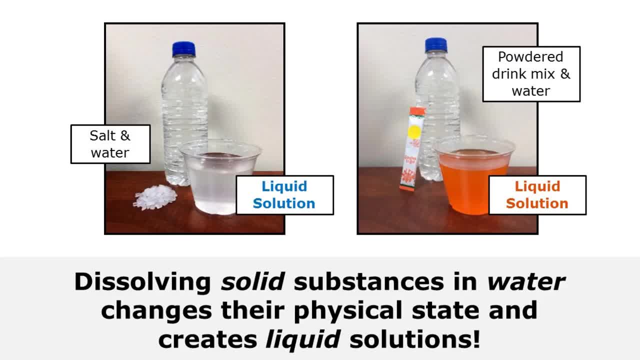 sugar water solution. Dissolving solid substances in water changes their physical state and creates liquid solutions. So the salt dissolves in the water and becomes evenly mixed with the water, And that salt takes on the physical state of the water and becomes part of a liquid solution. The same thing happens with the 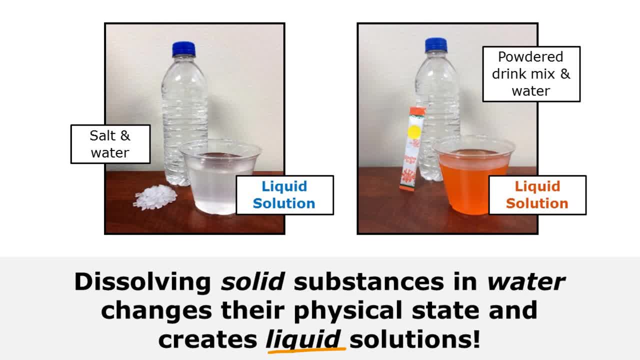 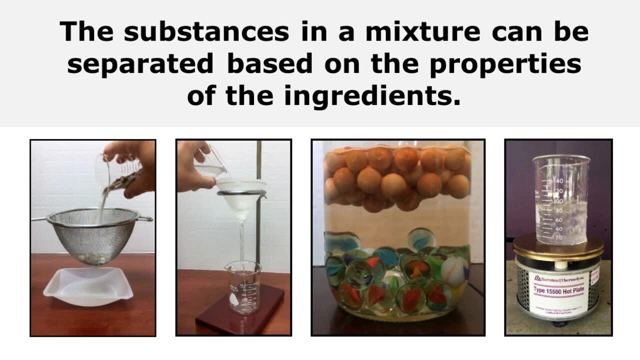 powdered drink mix. That powdered drink mix dissolves in the water and becomes a part of the liquid solution. Historical science has the里- I do not taste, ah reporter. water Во solution taking on the physical state of the water. The substances in a mixture can be separated based on the properties of the ingredients. 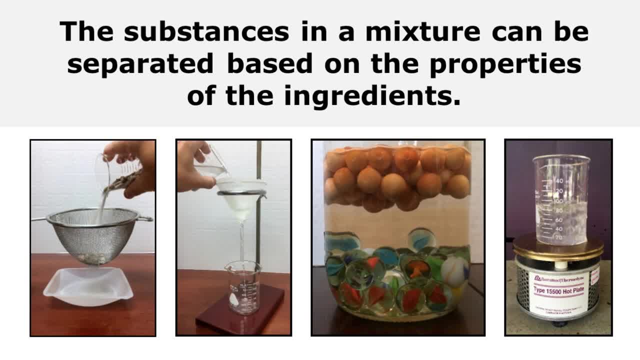 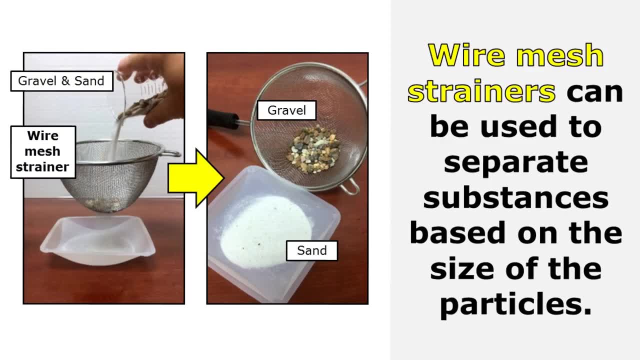 So it's important that you understand some of the basic methods that we can use to separate mixtures. Wire mesh strainers can be used to separate substances based on the size of the particles. So here you can see that I've got a mixture of gravel and sand and I'm pouring that through. 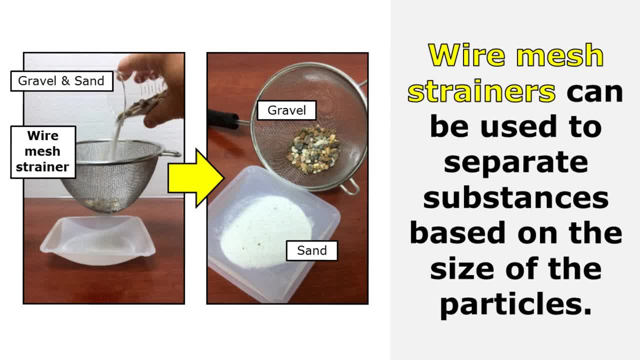 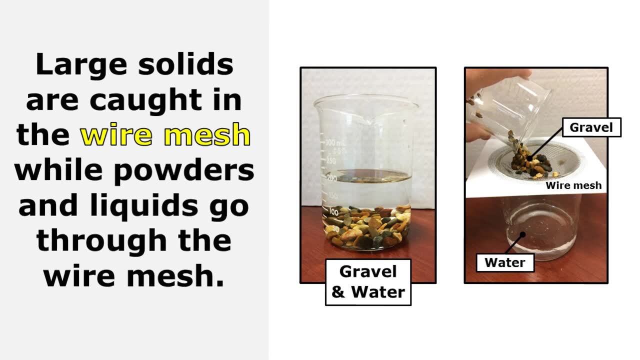 the wire mesh strainer. The grains of sand are small enough to go right through the wire mesh, but the gravel is caught in the strainer. So I'm able to separate this mixture because the size of the ingredients is different. Large solids are caught in the wire mesh while powders and liquids go through it. 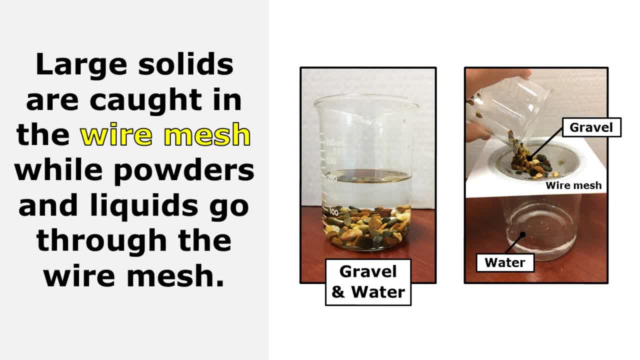 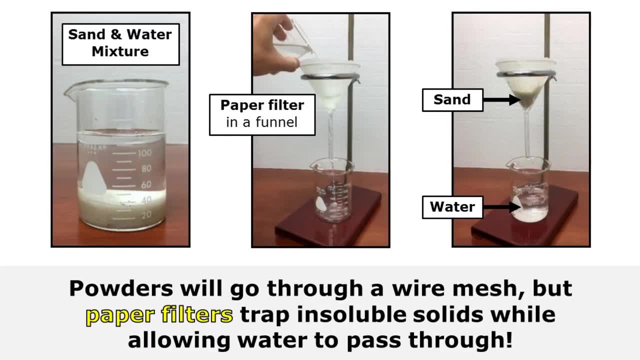 So here I have a mixture of gravel and water, and when I pour this mixture through the wire mesh, the gravel is caught by the wire mesh while the water goes right through. Okay, Let's see what happens. Powders will go through a wire mesh, but paper filters trap insoluble solids while allowing. 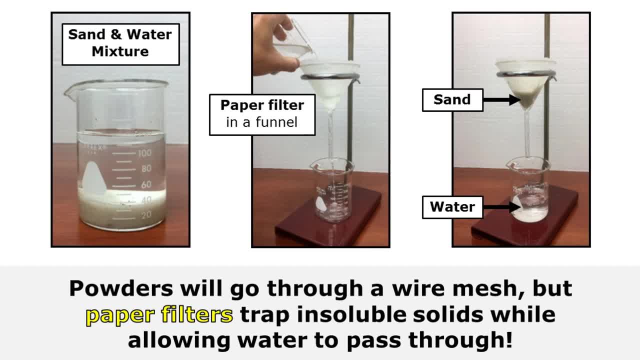 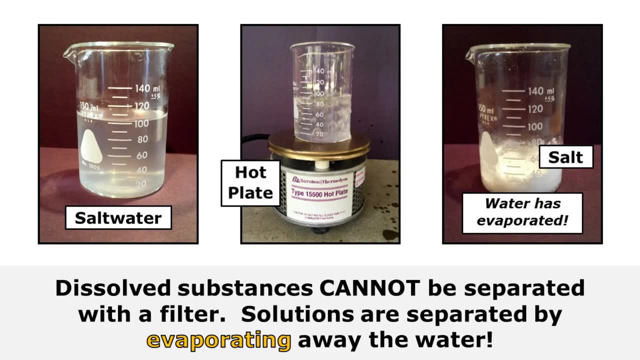 water to pass through. So here I have a mixture of sand and water. Now that sand would go through a wire mesh, but when I pour this mixture through a paper filter, the sand is caught by the paper filter while the water travels through. 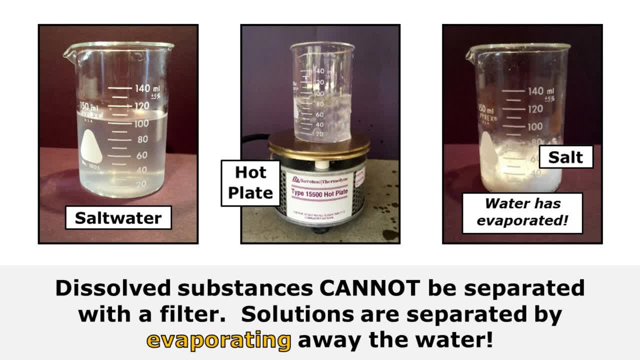 Dissolved substances cannot be separated. So here I have a salt water solution, a mixture of salt and water, but the salt has dissolved and become evenly mixed with the water. So I can't just pour this through a filter. the whole solution will go through the filter. 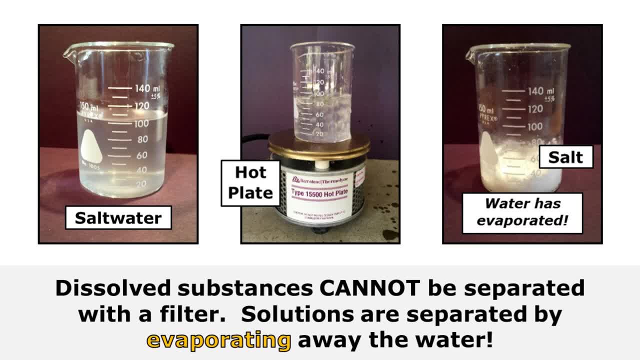 But I can put it on a hot plate and boil the water away. When I evaporate away all the water, I'm left with the salt and in that way I'm able to separate the salt from the water. So I separate the solution and get the salt away from the water. 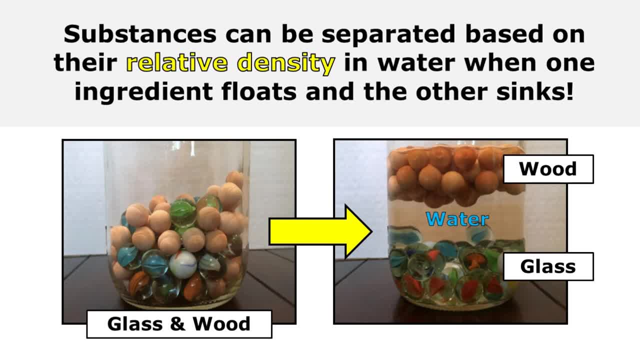 Substances can be separated based on their relative density in water, when one ingredient floats and the other sinks. So here I have a mixture of glass and wood, and I can separate this mixture pretty easily just by pouring water into this container. The wood will float to the surface of the water, while the glass sinks. 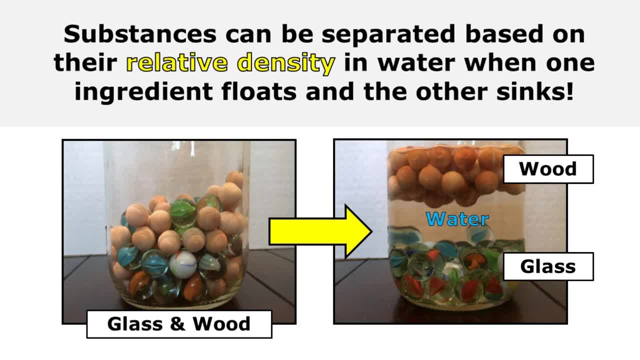 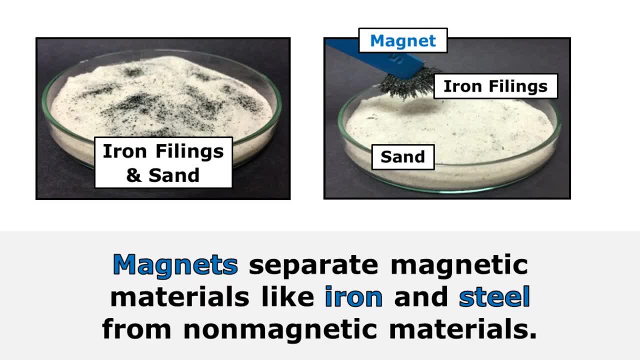 So, as you're thinking about how you might want to separate a mixture, it's important to think about the water. Also think about the physical properties of the ingredients, like their relative densities. Magnets separate magnetic materials like iron and steel from non-magnetic materials. 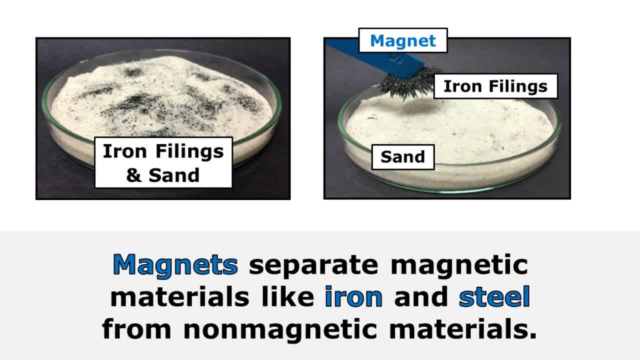 So here I have iron filings in sand and I can get those iron filings out of the sand by using a magnet. Once again, it's important to understand the physical properties of the materials that are in the mixture as you're trying to figure out how to separate that mixture.